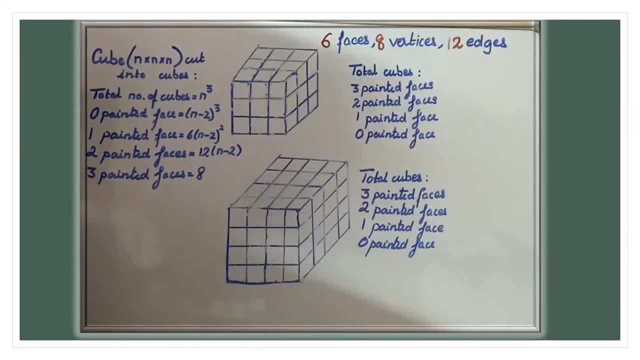 A cube has six faces, eight vertices and twelve edges. And if a cube is cut into smaller cubes, let's take this one here In this one, two, three. So it's length, three, And here one, two, three, width three, height one, two, three. 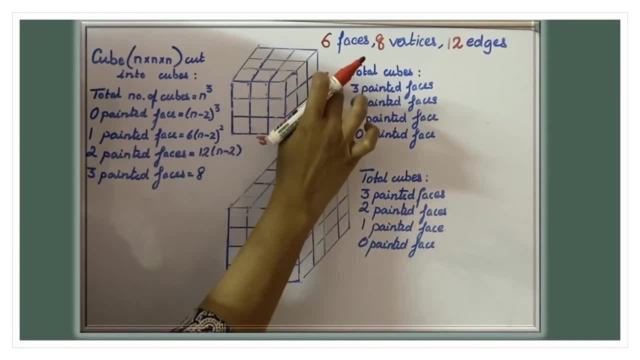 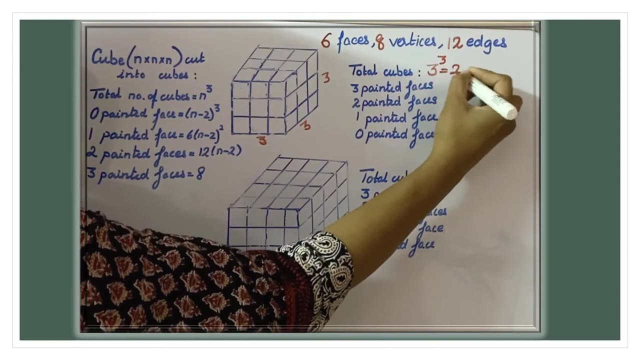 So this we can. we will say it as three into three, into three cubes. So the total cubes in this: if we cut this cube into smaller pieces, the total cubes we will get is n cube, n is here three, So which is three cubes. Twenty-seven smaller cubes are there in this cube. 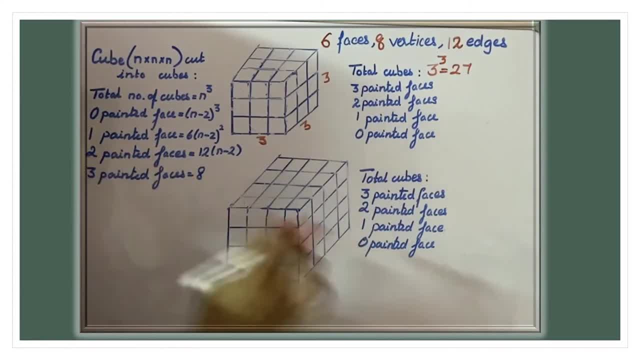 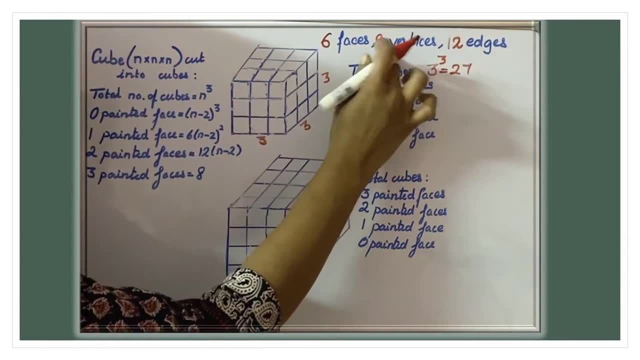 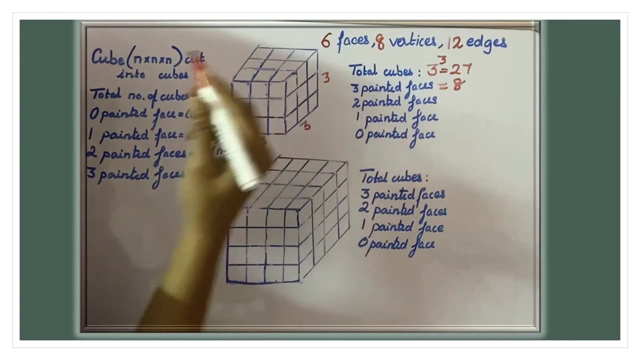 And how many cubes are three faces painted? To find three faces painted, look at the vertex. How many vertex are there in a cube? The cube has eight vertices. It means eight cubes. So eight cubes are three faces painted. That is only the cubes which is at the vertex. at each vertex will be three faces painted. 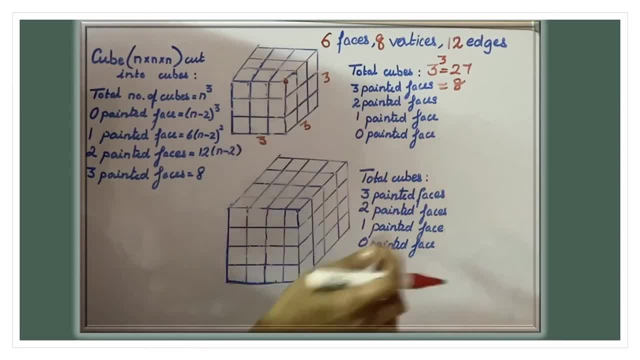 Here you can see one, two, three. This cube is three faces painted And in this vertex one, two, the bottom one is also painted. So three faces painted, Three faces painted. we can, we will get at each vertex. 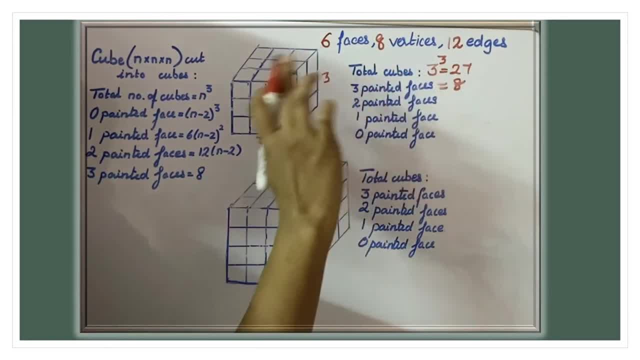 And how many vertex at the for cube Eight. So eight cubes are three faces painted. So out of twenty-seven, eight cubes are three faces painted. And how many cubes are two faces painted? Two faces painted, you will get at edge. 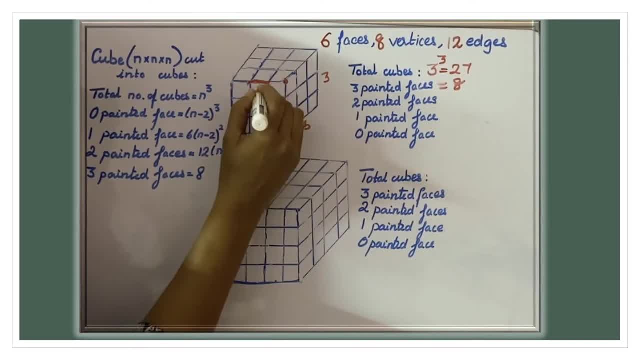 See, in this edge, this cube, this cube is two faces painted, One here, one here. This is two faces painted, Two faces painted. So how many cubes are? two faces painted means the cube which is at the edge. Take the edge. 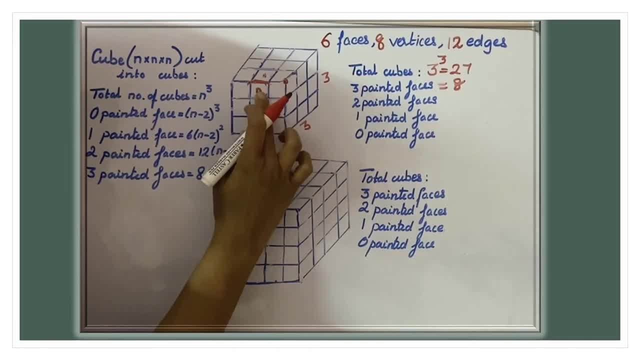 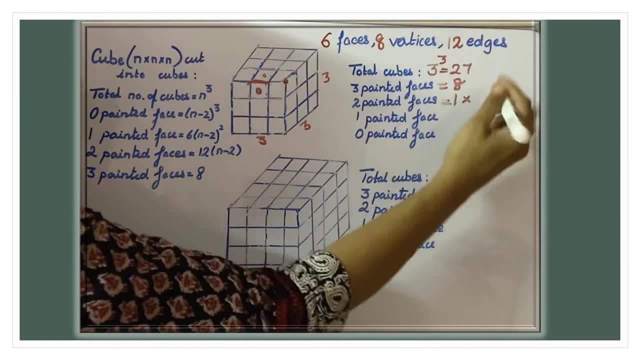 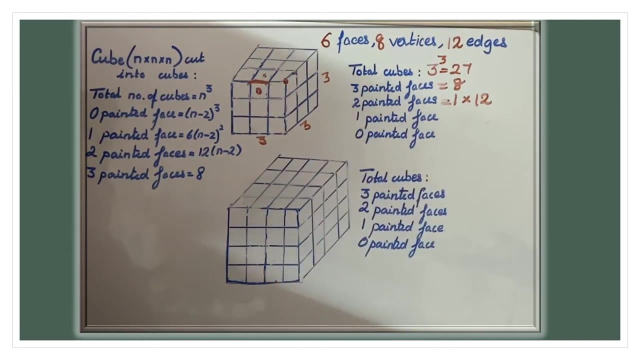 Each edge in this edge, how many cube? Only one cube. Take that one, multiply with how many edges for the cube: Twelve edges. So it means that twelve cubes are two faces painted. Next, how many cubes are one faces painted? 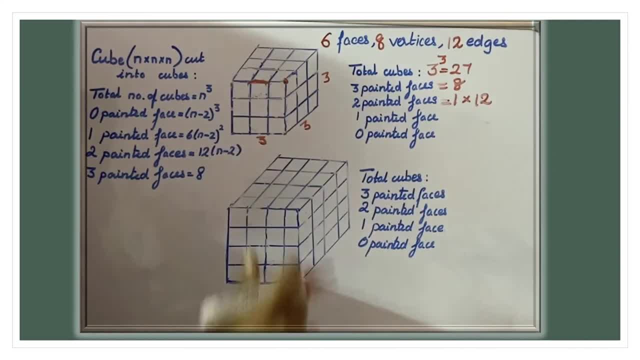 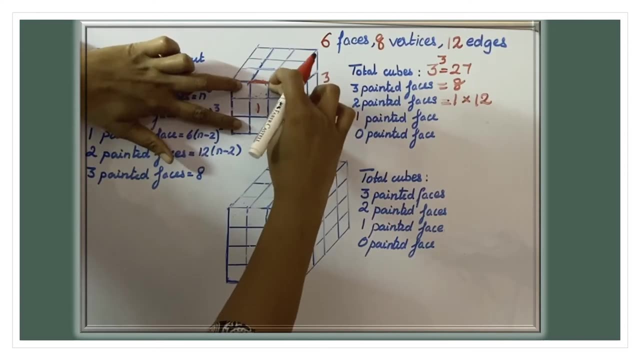 For one faces painted. take the face, This is a face right In this face. how many cube is one face painted? Only this cube is one face painted. See this, two cubes are three faces painted. This, sorry, the corner one. 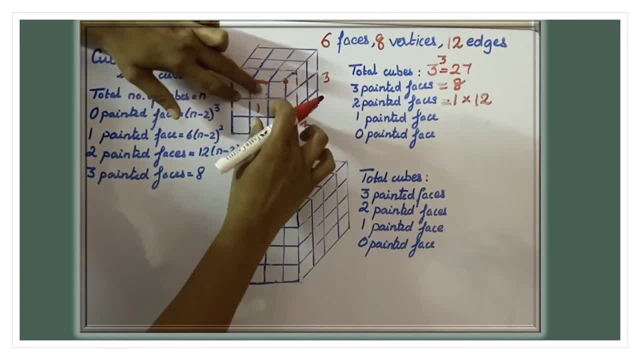 This four cubes are three faces painted And this, this, this, this is, these are two faces painted, Reminding only this cube is one face painted. So how many cubes for a face In one face? how many cube is one face painted? 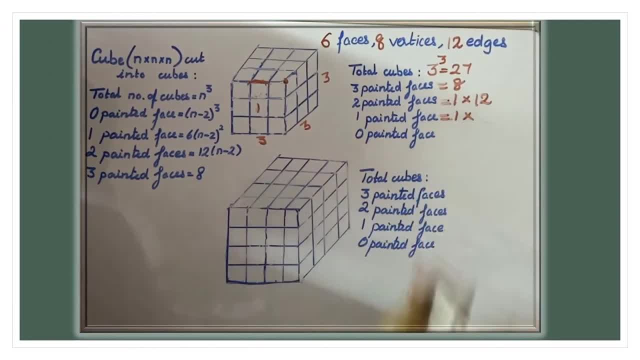 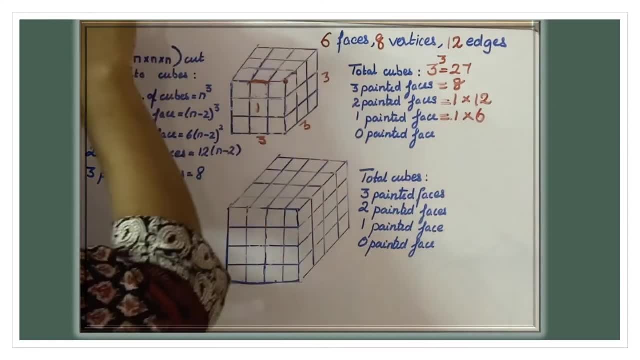 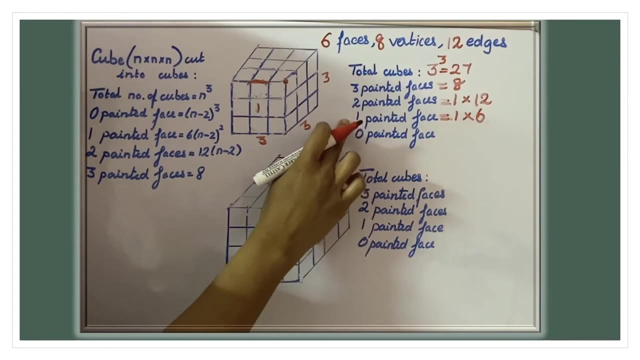 One. Take that And a cube has how many face? Six. So like this we will get one more here, One more here And three at the hidden one. So one into six. there are six cubes which are one face painted. 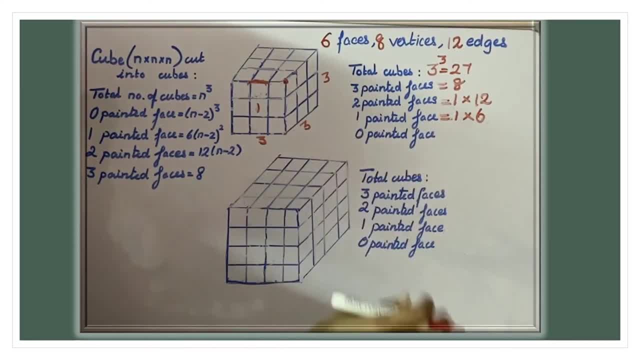 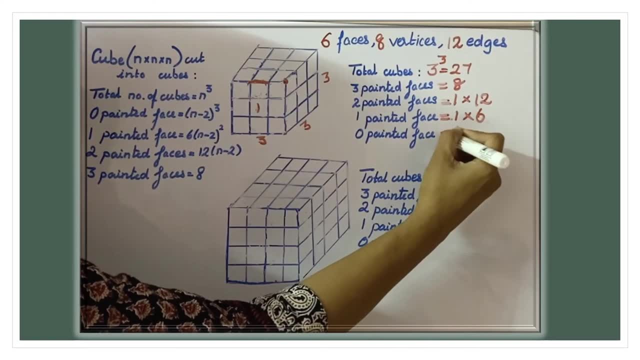 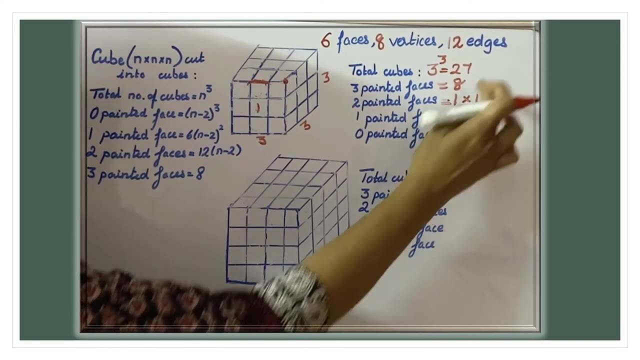 Next, how many cubes are zero face painted? Zero faces painted is the cube which is at the middle layer, At the middle layer, middle cube, is zero face painted. And now, if we add this, one eight plus twelve, which is twenty plus six, twenty six plus one twenty seven, 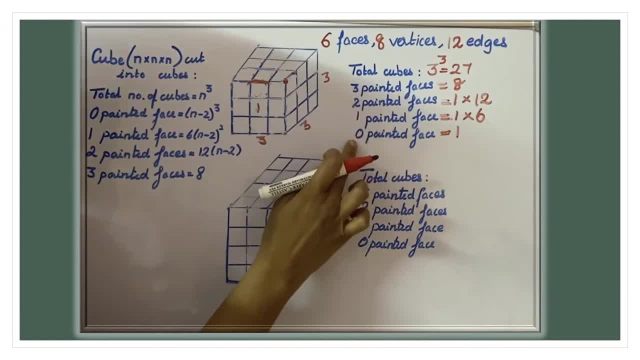 This is the total cubes. If we add this, three face, two face, one face and zero face painted cubes, we will get the total cubes. That's it. Now let's check this one. And here it's: one, two, three, four. 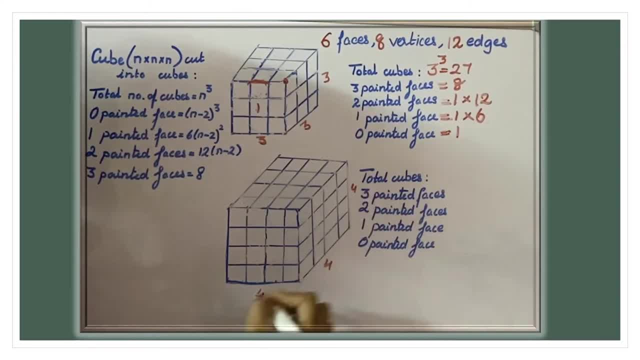 So this is four and four, four. This is four into four, into four cubes. So n is four, And let's see how many smaller cubes are there in this. So which has four cube is sixty four cubes are there. 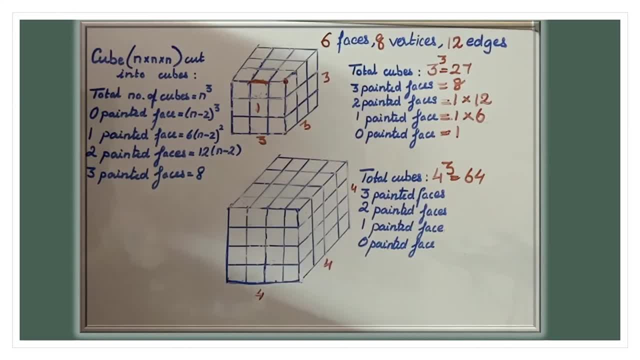 Fifty, sixty four smaller cubes are there in this, And let's see how many are there. Three faces painted. Three faces painted are always same for whatever it is: Three into three, or four, into four or five, into five cubes. Three faces painted means it's eight. 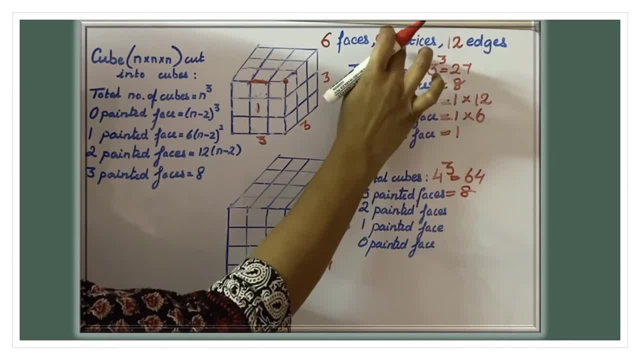 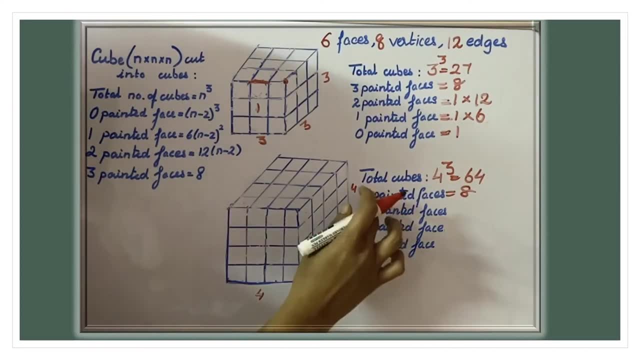 It's same for all, Because there are eight faces, eight vertices, a cube as So at each vertex we will find a cube with three faces painted. And how many vertices? Eight vertices, So there are eight cubes with three faces painted. 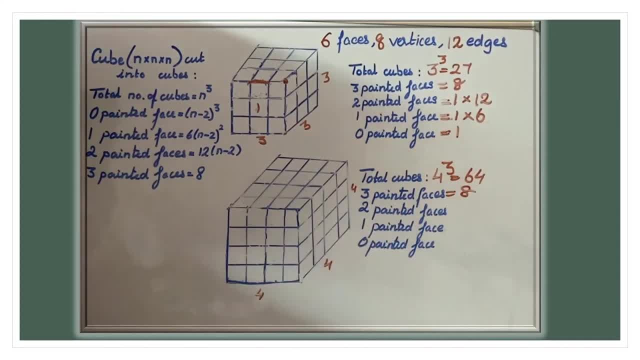 That's it. Come for this. Two faces painted. How many are two faces painted? Let's check that. Two faces painted means we have to look at the edge. So in this edge- let's check this edge- How many are two faces painted? 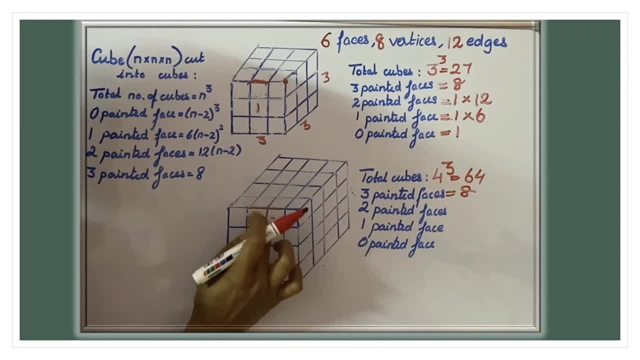 Only these two. See, this is two faces painted. So these two, So how many cubes? Two And how many edges? Twelve Multiply. If you multiply this, we will get How many cubes are two faces painted? 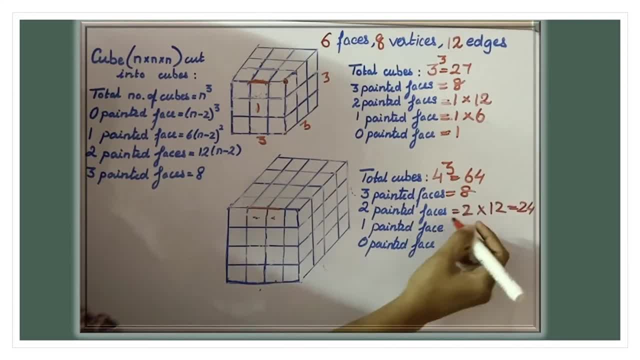 So total is 24 cubes. are two faces painted, Next single face painted, Single face painted. is this: These four, These four cubes are single face painted. So in this one face, in one face four cubes. So totally, how many faces are there? 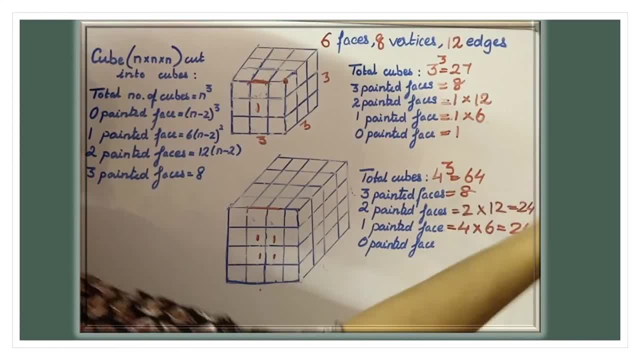 Six faces, So total four into six. 24 cubes are single face painted in this. Next: zero face painted. Zero face painted cubes For zero face painted cubes. look at the middle layer In this. look at the middle layer. 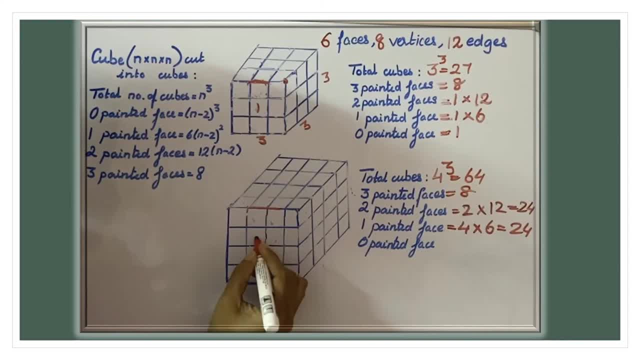 That is, leave this and this, Take the middle. In this middle layer there are four cubes, So four. Take this four In this middle layer: one, two, three, four cubes And in this also take the middle. 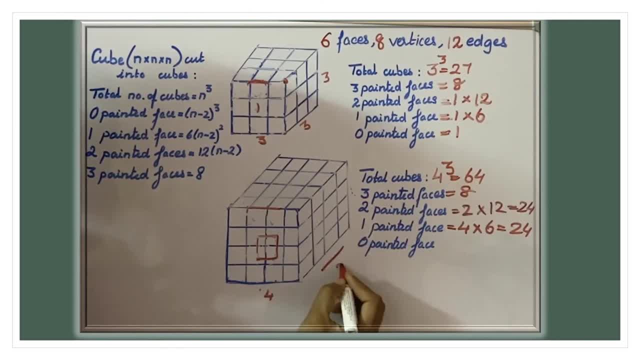 Leave these two and take the middle, How many? Two. So it means four into two. We have to do four into two. Four into two, which is eight, Eight cubes are zero face painted. And if we add these three face, two face, single face and zero face painted. 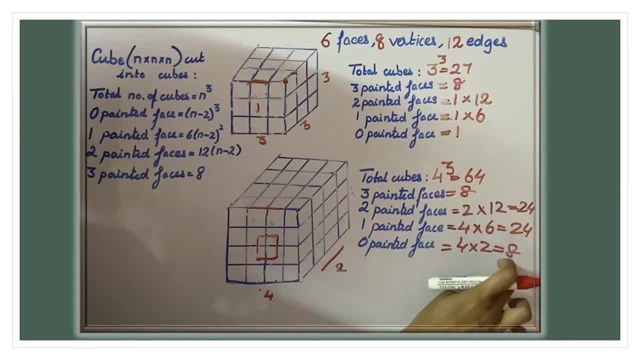 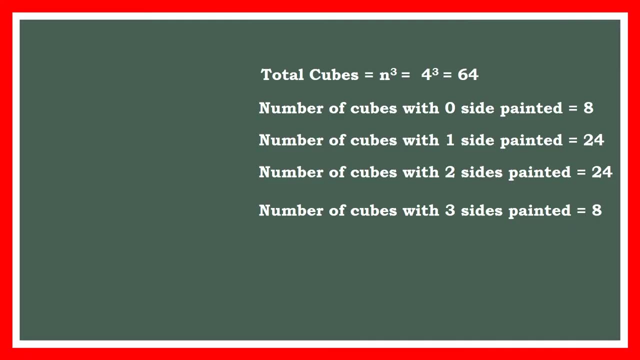 Eight plus twenty-four, which is thirty-two plus twenty-four. fifty-six plus eight, sixty-four: That's the total cubes in this. That's it. Total cubes in this. That's it, That's it, That's it. 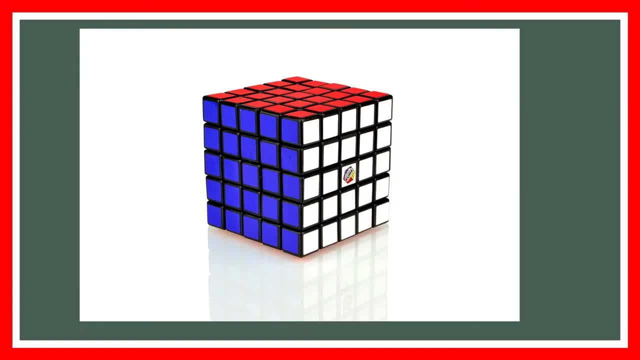 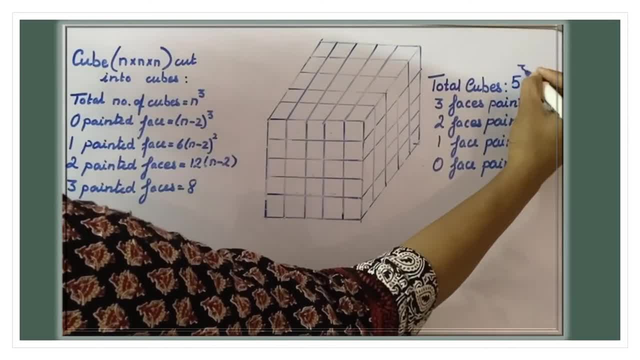 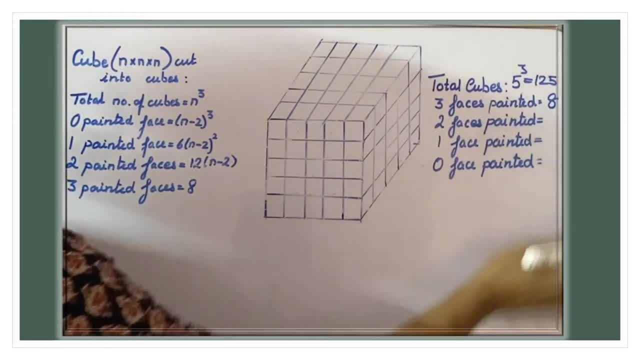 And how many cubes are three faces painted? Eight smaller cubes are three faces painted. This remains same. And how many are two faces painted? For finding out these, we can use this formula: or, for two faces painted, just check the edges At this edge. 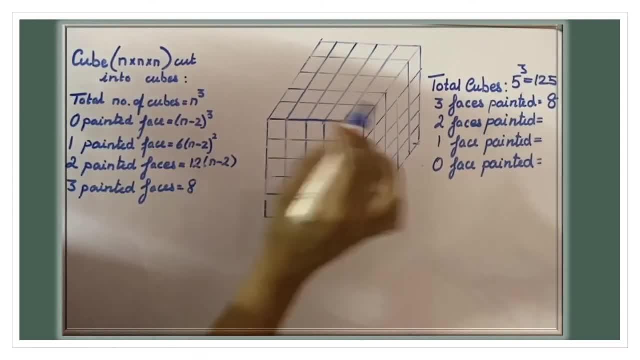 At one edge. how many cube is? two faces painted, Just check for one edge. How many faces are painted? Just check for one edge At this edge, one, two, three. So these three cubes are two faces painted, Two faces painted. 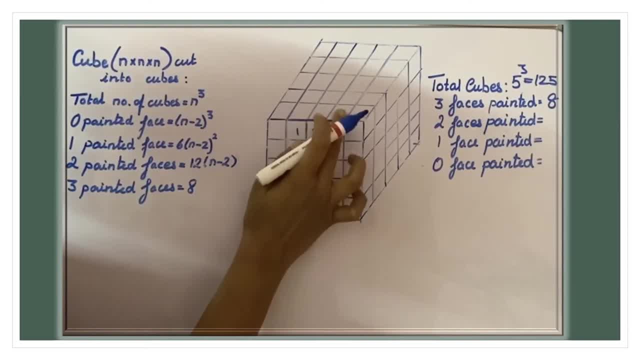 So three into how many edges? totally Twelve. So it means three into two. twelve. Thirty-six smaller cubes are two faces painted. You can find by the formula or just check: take one edge and at one edge how many cubes. 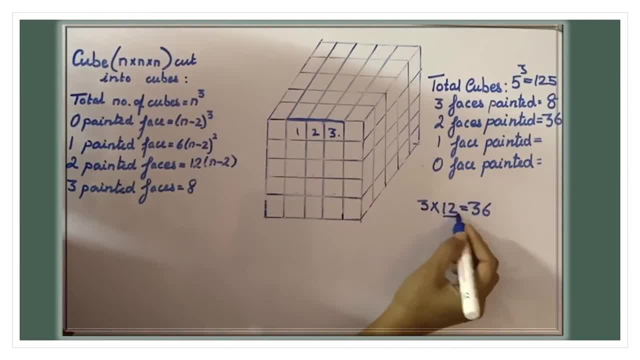 are two faces painted. Check that and multiply with the total edges. Next, how many is single face painted? For single face painted: again, you can do by formula or for single face painted, what we can do: take us one, any one face, any one face, and check in that how many are single. 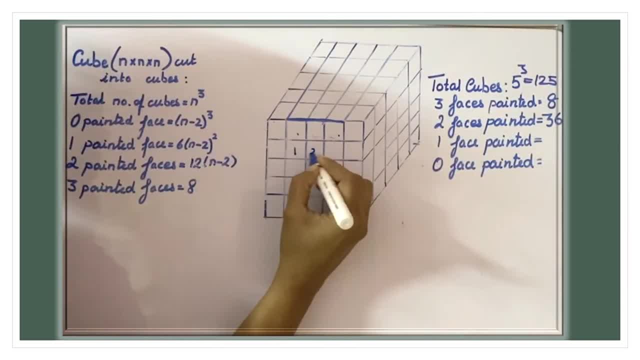 face painted, The cube here, this one, this, these cubes are single face painted. So totally, how many Nine. So nine smaller cubes in one face, In this one face. nine cubes are there. So totally, how many cubes faces are there. 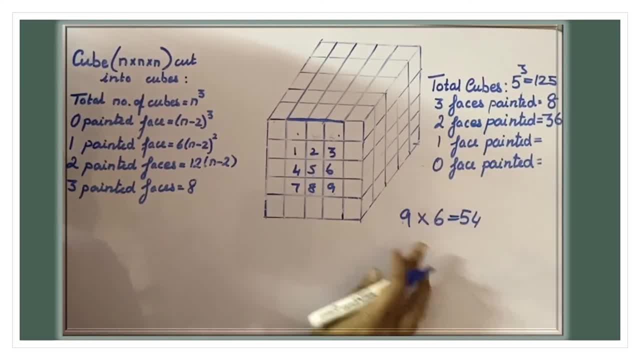 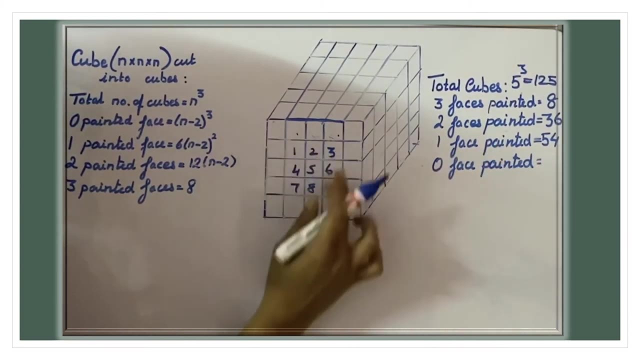 Six faces. So it means that fifty-four smaller cubes are single face painted. Next, how many zero face painted For zero face painted here? take this one, this nine We have already found you know for single face. take this nine. 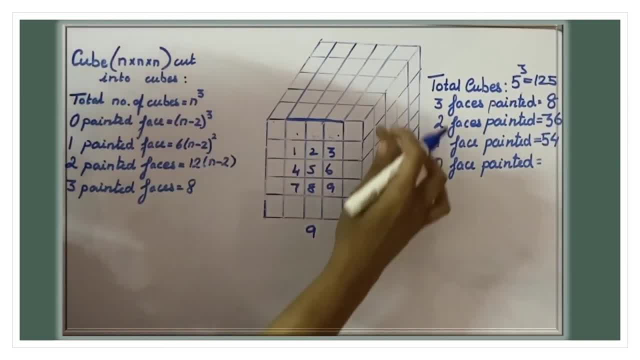 Okay, And here we have to check the layers, because the middle layer only will not be painted. So the middle layer, middle layer, is how many? Leave this and this And take this one, two, three, So it means middle layer, middle. there are three layers.